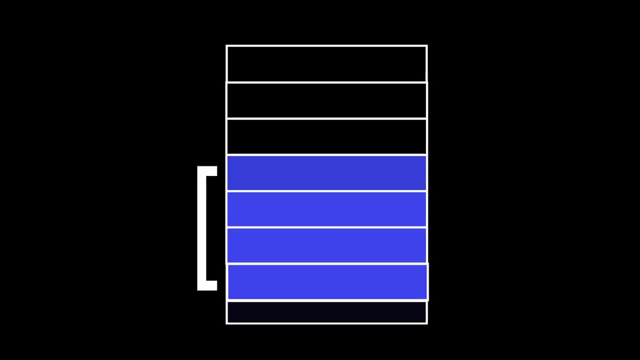 the virtualization technique dynamically replaces the rendered items with new ones. Here we have a list of items that are currently visible within the viewport, thereby conserving resources. As the user scrolls through the list, the virtualization technique keeps the visible portion of the list updated and responsive. It allows you to efficiently 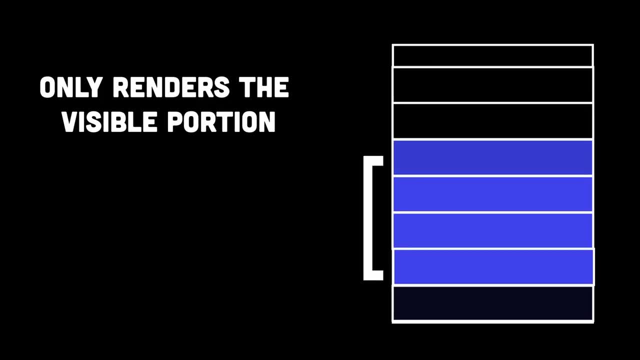 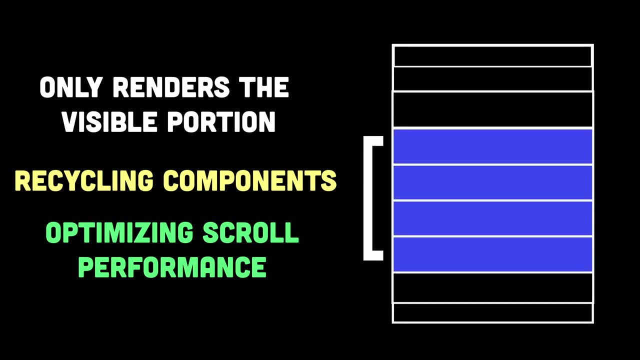 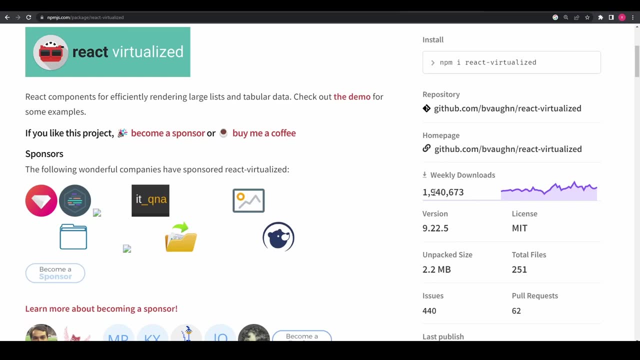 render large lists or tabular data by only rendering the visible portion, recycling components as needed and optimizing scroll performance. There are different approaches to implementing list virtualization in React. One popular library that provides this functionality is React, Virtualized By leveraging list virtualization. React applications can handle. 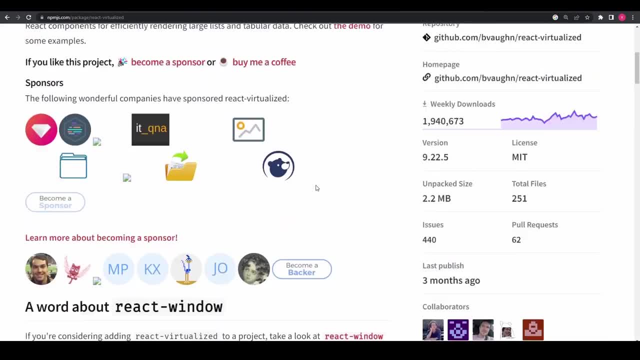 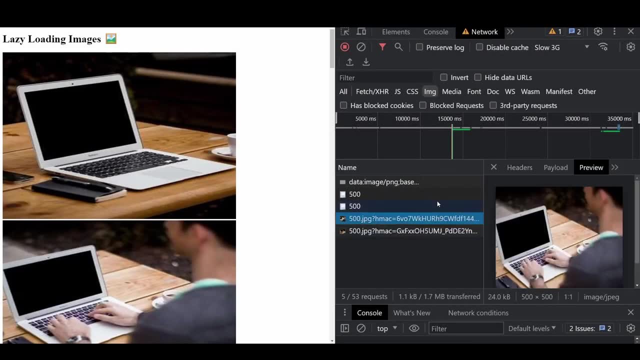 massive amounts of data without sacrificing performance or user experience. In number 2, we have lazy list virtualization. In number 3, we have lazy list loading images, Similar to the list virtualization technique mentioned in number 1, lazy loading images prevents the creation of unnecessary DOM nodes, thereby boosting performance. 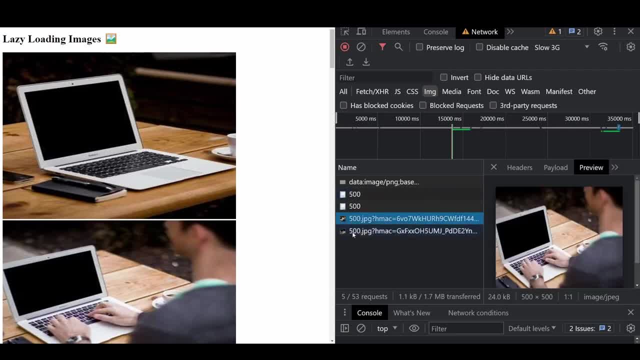 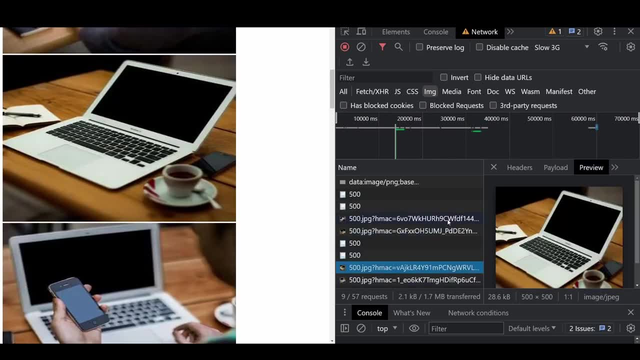 So with lazy loading, instead of loading all the images on page load, lazy loading allows you to defer or delay the loading of images until they are actually needed or visible to the user. The concept behind lazy loading is to initially load a placeholder or a small 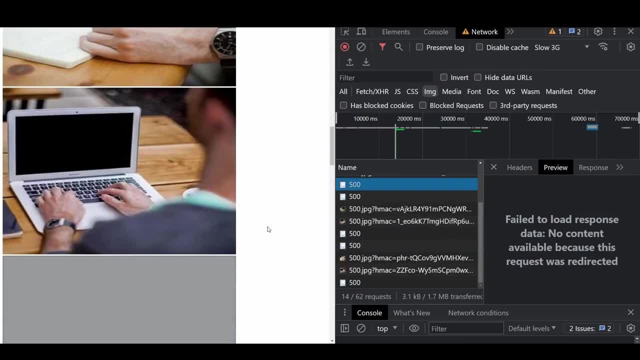 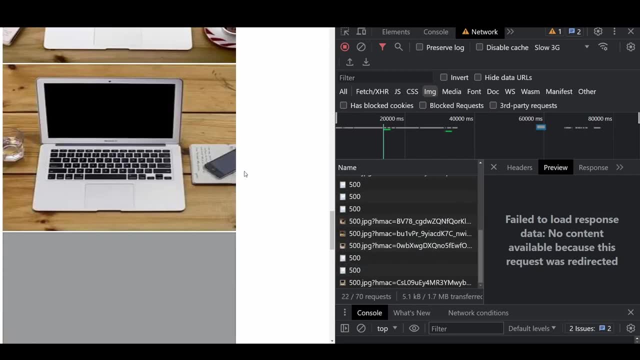 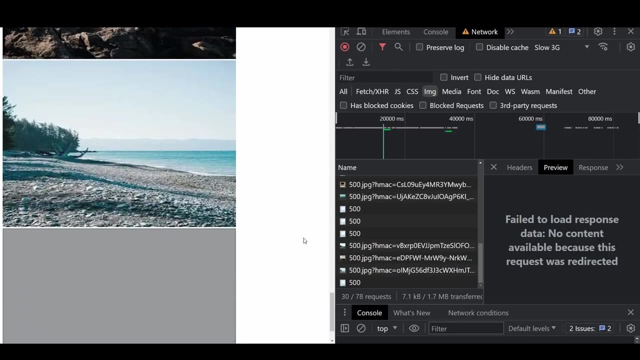 low-resolution version of the image, typically a small-sized thumbnail or a blurred placeholder. As the user scrolls or interacts with the page, the actual image is loaded dynamically, replacing the placeholder, only when it enters the viewport or is about to become visible. Lazy loading images in React can be achieved using various libraries and techniques. 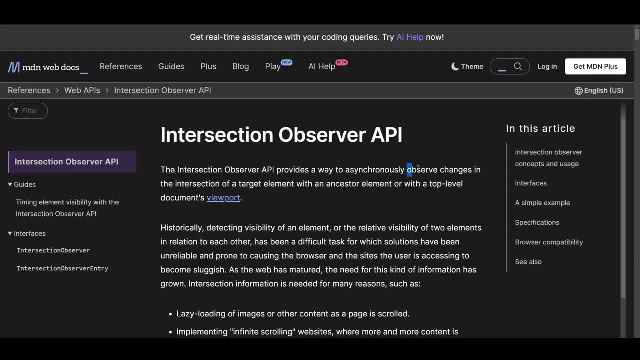 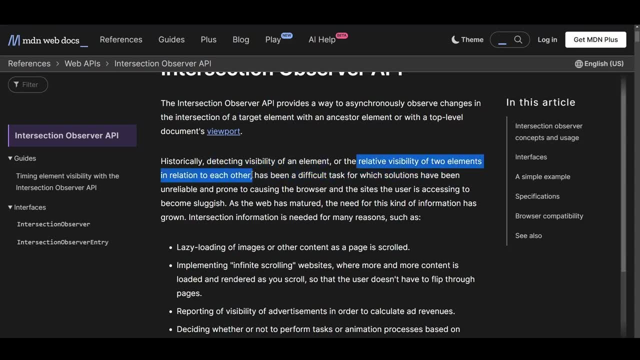 One popular library is React Lazy Load. Another approach is to use the Intersection Observer API, a web API that allows you to efficiently detect when an element enters or exits the viewport. By utilizing this API along with React's useEffect hook, you can implement your custom 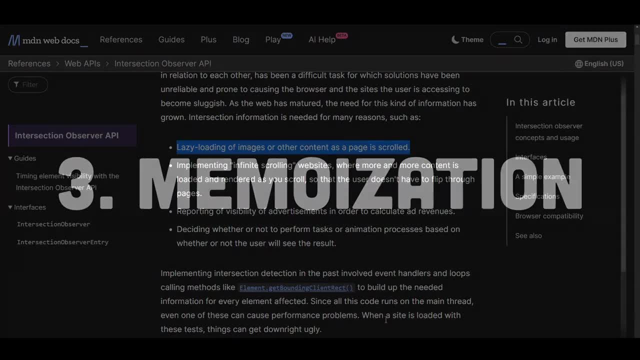 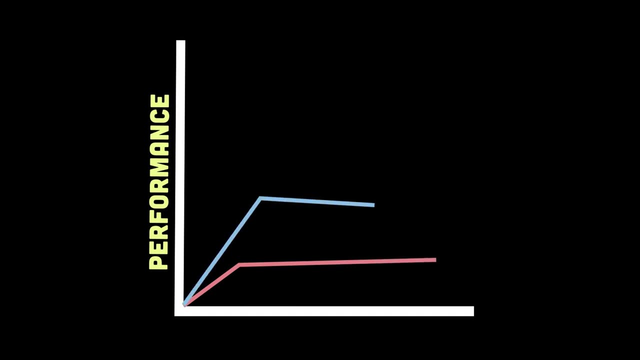 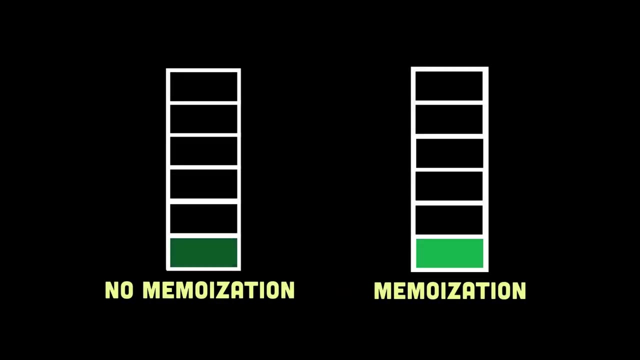 lazy loading solution for images in React. 3. Memoization: Memoization in React is a technique used to optimize the performance of function components by caching the results of expensive computations or expensive function calls. It is particularly useful when dealing with computationally intensive, or frequently called, functions. 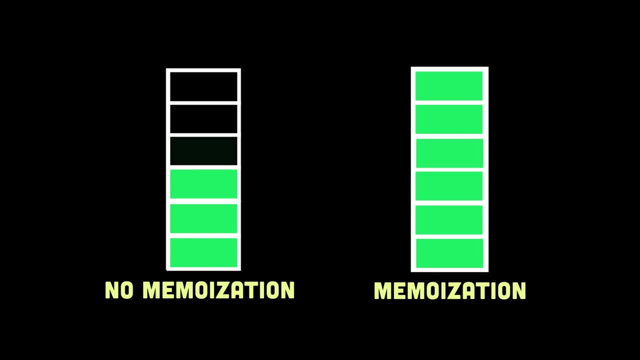 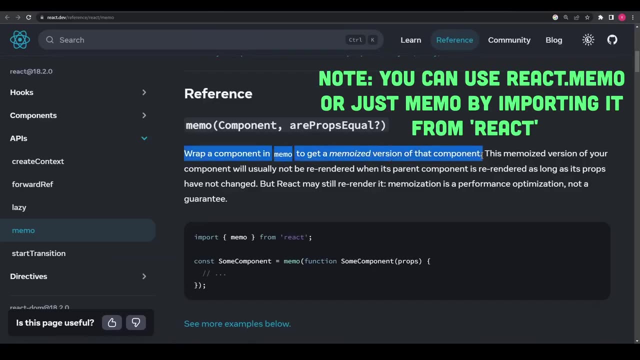 that have the same input values, as it helps avoid redundant calculations and improves the overall efficiency of the application. In React, there are three techniques for memoization: 1. ReactMemo, 2. UseMemoHook, 3. UseCallBackHook. ReactMemo is a higher-order component used to wrap a purely functional component to prevent 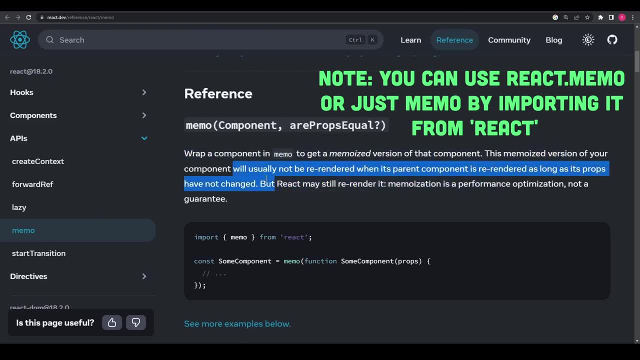 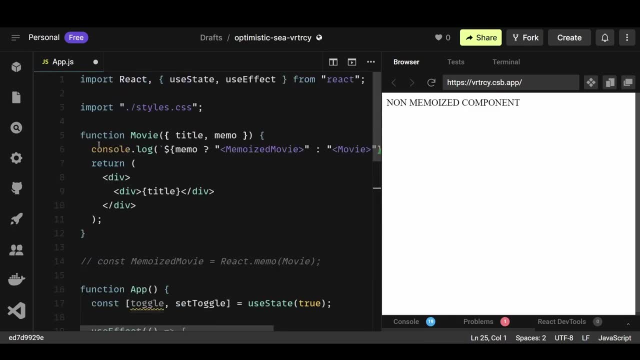 re-rendering if the props received in that component never change. Imagine you have a function component that renders some content based on its props. Normally, whenever the component's parent re-renders, the component itself would also re-render, even if the props 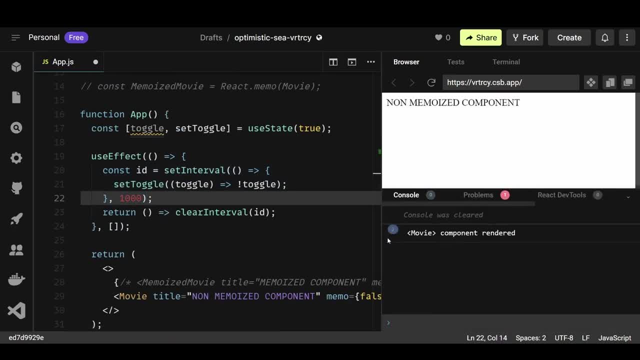 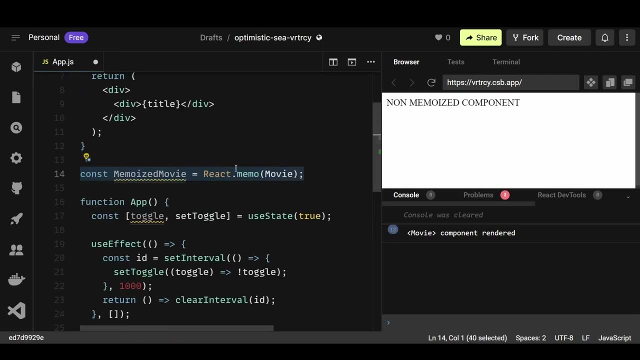 haven't changed. This can be inefficient if the rendering process is computationally expensive. By wrapping your component with ReactMemo, you can re-render the props that you received in the component. React remembers the result of rendering the component based on its props. 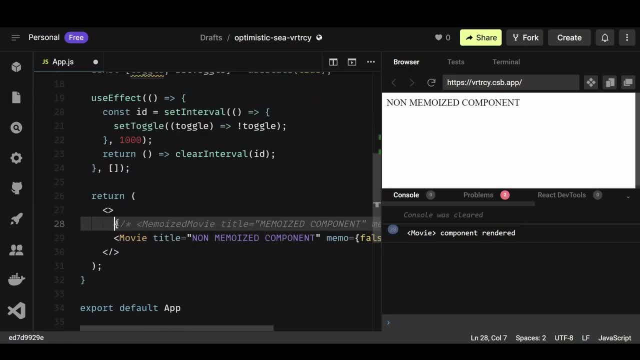 If the props haven't changed since the last render, React will reuse the previously rendered result instead of re-rendering the component from scratch. This saves time and resources. In other words, ReactMemo helps prevent unnecessary re-rendering of components when the props remain the same. 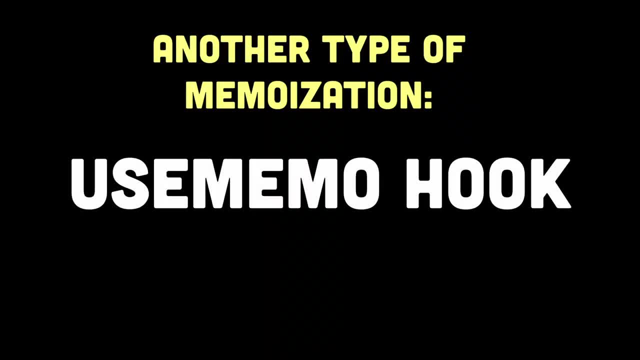 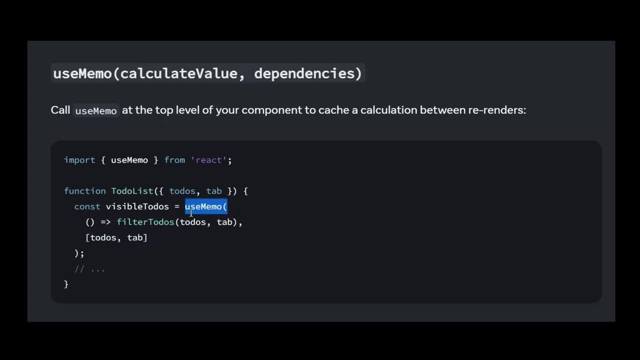 Then we can have another type of memoization in React, which is the UseMemoHook. The UseMemoHook in React is a way to optimize performance by memoizing the result of a function or an expensive computation. Imagine you have a function that performs a time-consuming 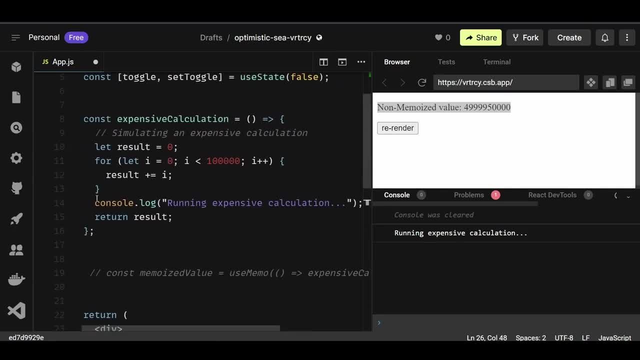 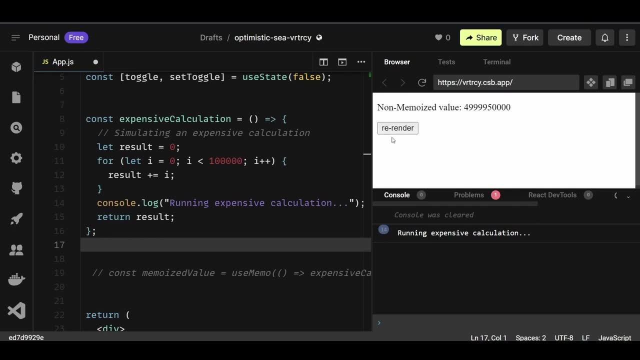 calculation. Normally, this function would execute every time your component re-renders, even if the input values haven't changed. This can lead to unnecessary computations and impact performance. By using the UseMemoHook, you can tell React to remember the result of the function. 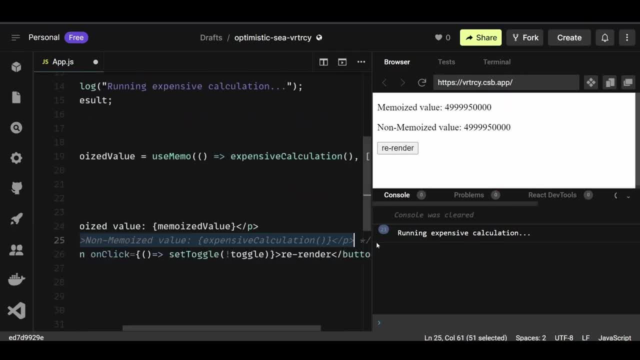 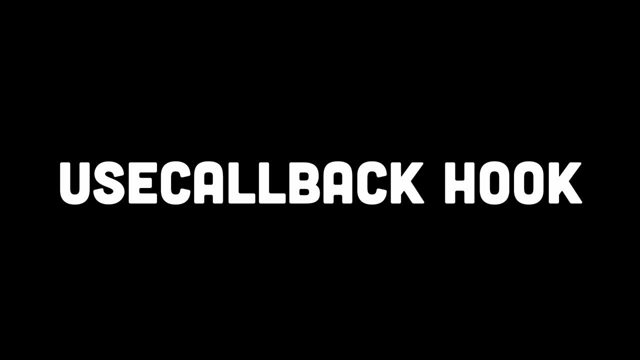 call and only re-calculate it when the input values change. It caches the result and returns it whenever those input values remain the same. Then we can have the third type of memoization, which is the UseCallbackHook. The UseCallbackHook in React is used to optimize the performance by memoizing a function instead. 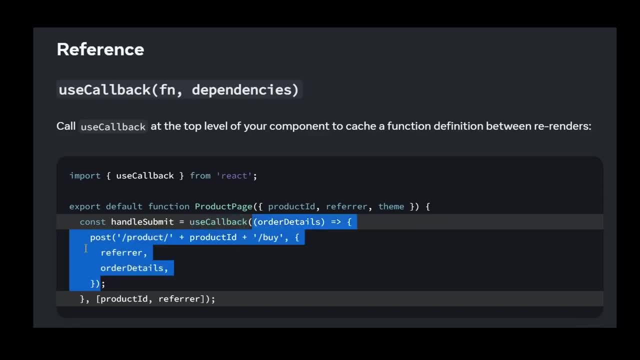 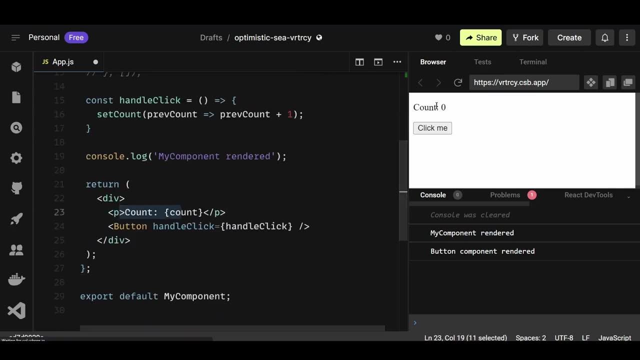 of memoizing the function result. like UseMemo does, UseCallbackHook is particularly useful when passing function as props to child components, as it helps prevent unnecessary re-renders In React. when a component re-renders, all functions defined within it are recreated. 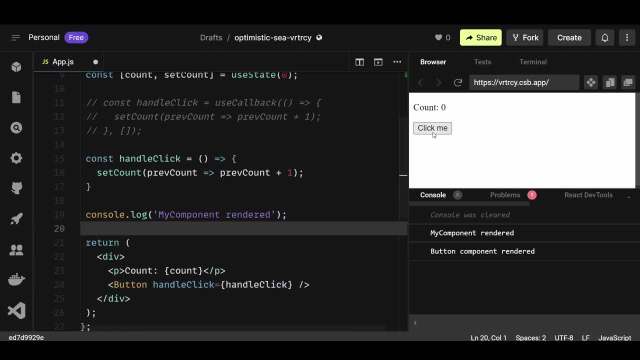 This means that every time a parent component re-renders, the child components which take functions as props receive new instances of those functions from the parent component. The child components receive new instances of the parent component even if the functions haven't changed. This can lead to unnecessary re-renders in child components because it thinks its props. 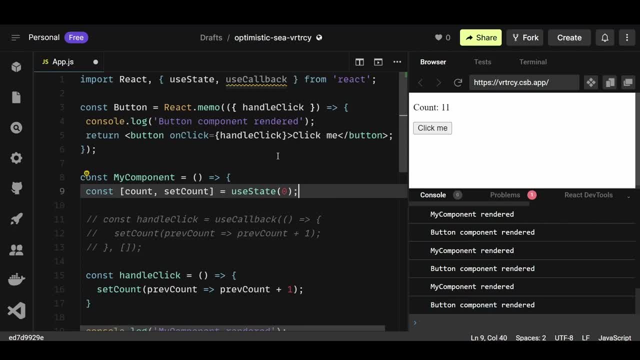 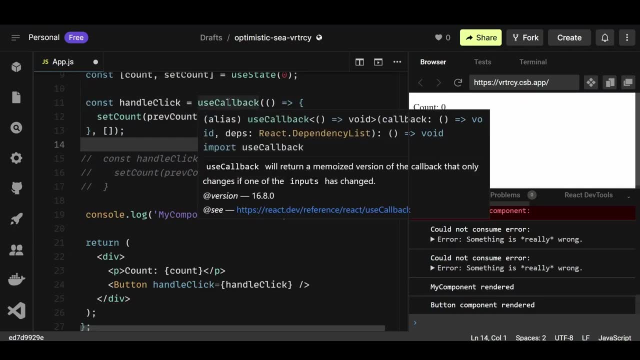 have changed, thereby impacting performance. By using the UseCallbackHook, you can memoize a function and ensure that it remains the same between re-renders as long as the dependencies haven't changed. This way, child components that receive the function as a prop won't re-render. 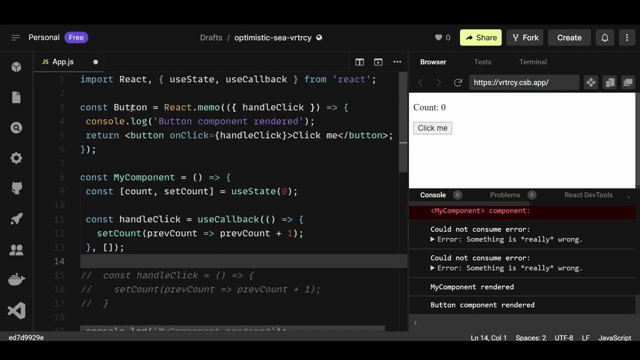 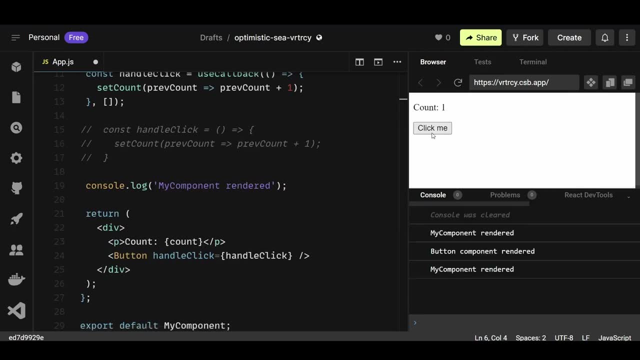 unnecessarily when the parent re-renders. UseCallback is often used with ReactMemo because ReactMemo will ensure that a re-render is not a result of a child component re-rendering a function. A re-render in the parent component doesn't re-render the child component if the props 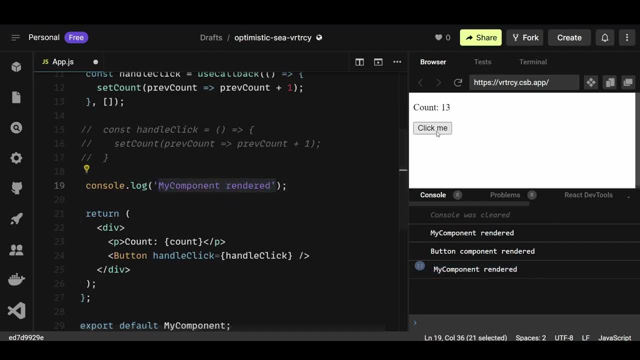 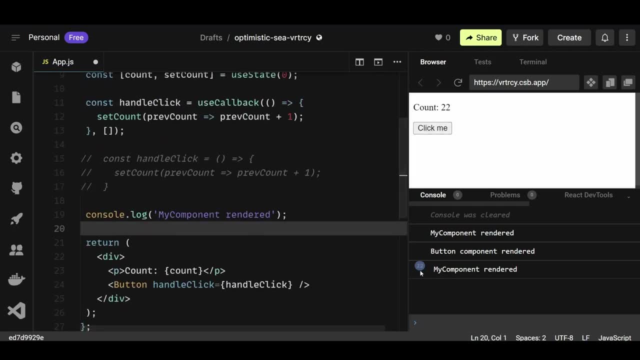 haven't changed, and UseCallback will make sure to stop the re-creation of a new function instance during every re-render, allowing that function being passed as a prop to a child component to be the same instance across re-renders, ultimately allowing the child component to not re-render at. 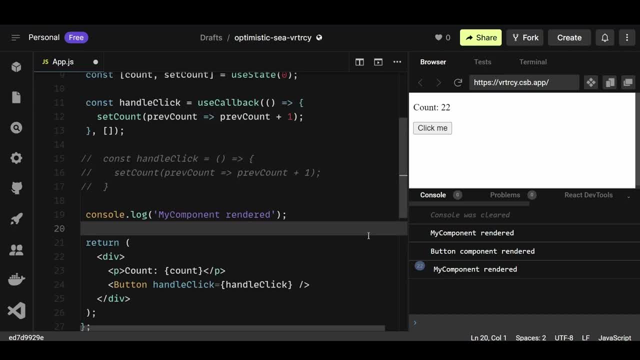 all, even when functions are passed as a callback. So that's why ReactMemo and UseCallback are often used together. If you found this difficult to understand, then comment down and I'll make a video on this, explaining everything step by step in great detail. 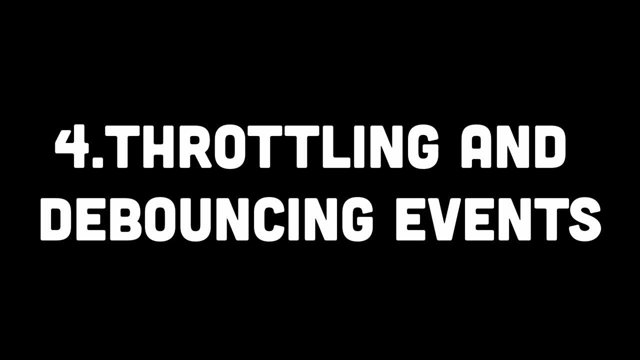 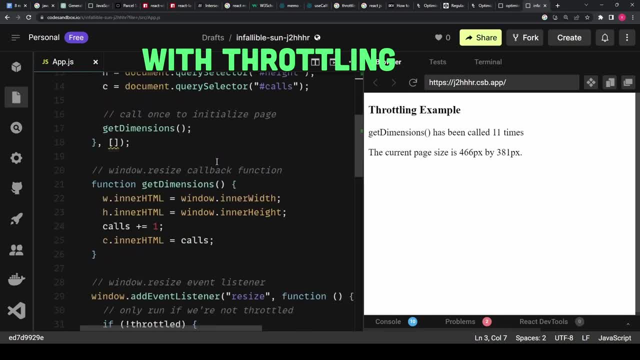 Now in number 4, we have Throttling and Debouncing Events. Throttling in React is a technique used to limit the number of times a function or an event handler is invoked. It ensures that the function is called at a specified interval. 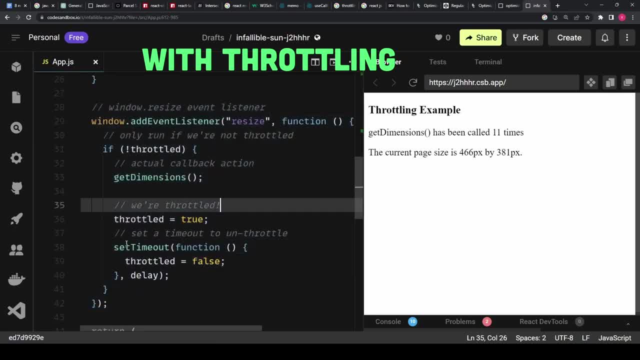 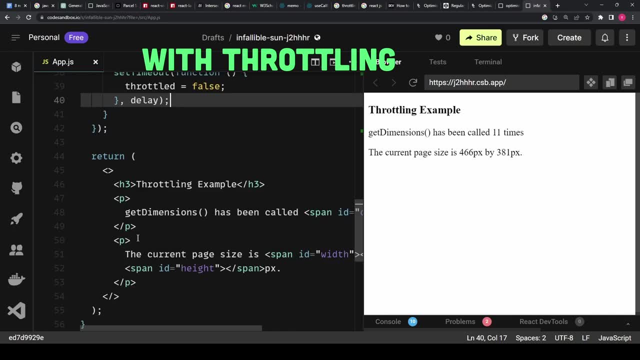 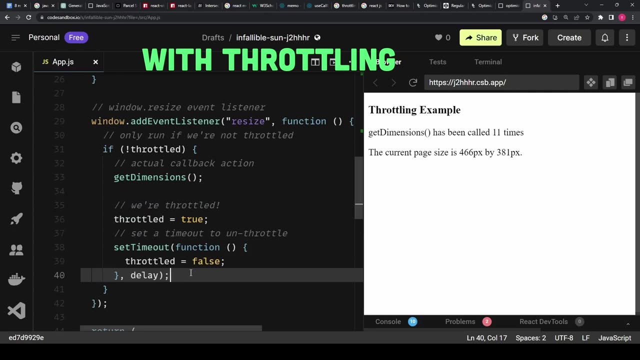 preventing it from being executed too frequently. Throttling allows you to control the rate at which the function is called by setting a minimum time interval between every function invocation. If the function is called multiple times within that interval, only the first invocation is executed and subsequent invocations are ignored until the interval elapses. 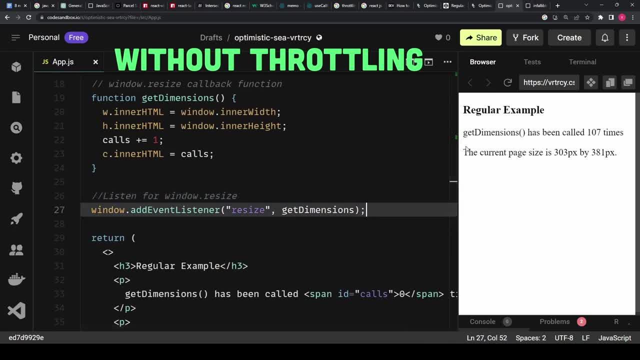 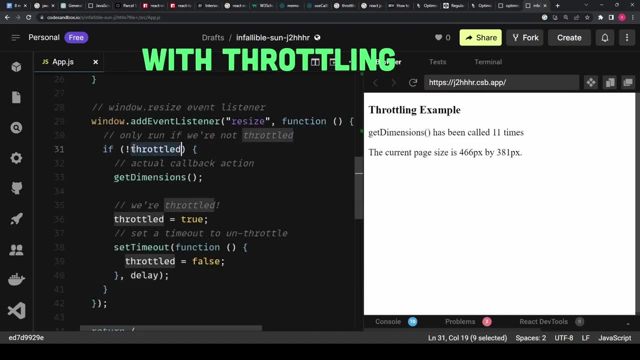 For example, let's say you have a window resize event handler that triggers a function to perform some calculations or update the UI. By applying throttling you can ensure that the function is called, let's say, every 200 milliseconds, If the user resizes the window rapidly. 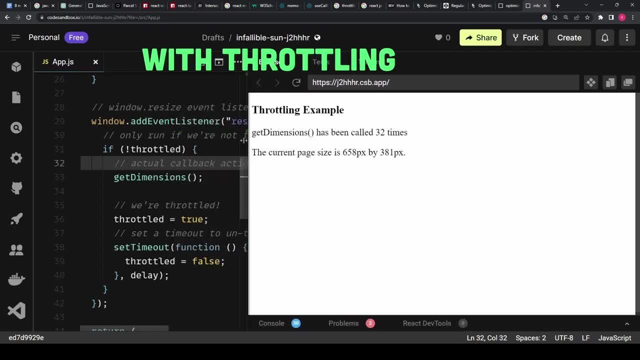 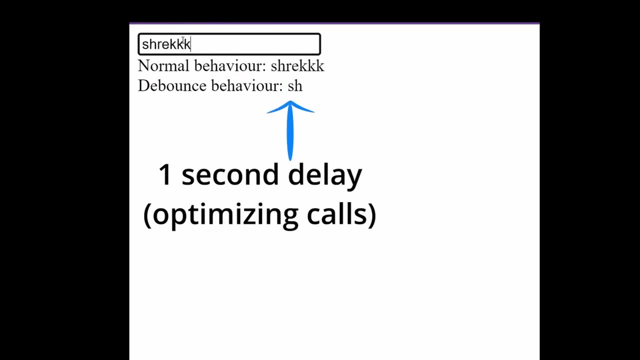 the function will be invoked at most once every 200 milliseconds, instead of being invoked every time the window was resized, reducing the number of computations or UI updates and improving the functionality. The function is called only after a certain period of inactivity, delaying the function execution until a pause in the event stream occurs, such as pausing after. 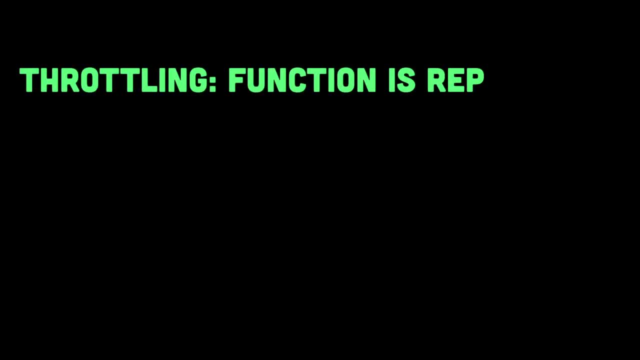 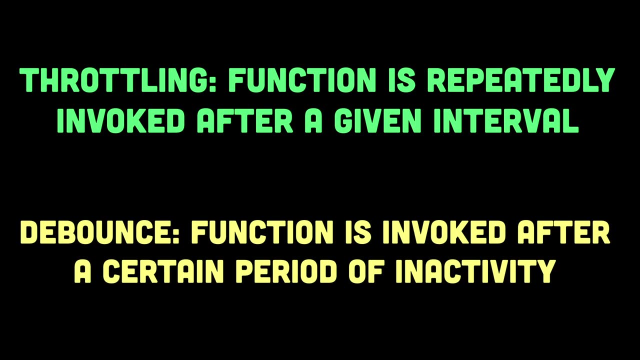 typing in an input, making it different from throttling, where the function was repeatedly called after a given interval. So debouncing allows you to postpone the function call until the user has finished typing or a specific time has elapsed since the last event. For example, let's say: 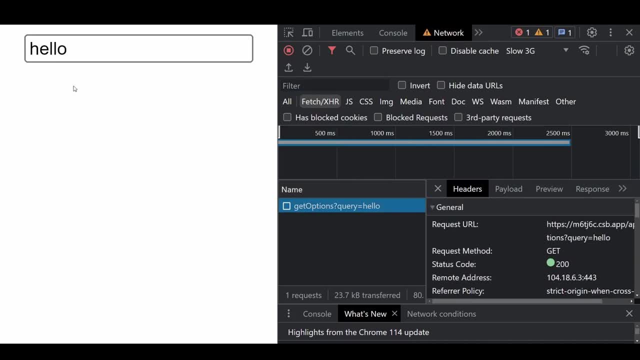 you have a search input field and you want to trigger a search API request only when the user has finished typing for a certain duration, like 300 milliseconds, With debouncing. the search function will only be invoked after the user stops typing for 300 milliseconds. If the user 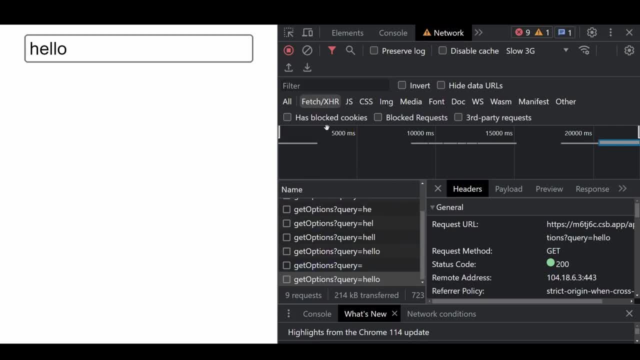 continues typing within that interval, the function call will be delayed until the pause occurs, Whereas without debouncing the function would be called for every key stroke, potentially leading to excessive function calls and unnecessary computations. Now, in number 5,, we have code splitting. 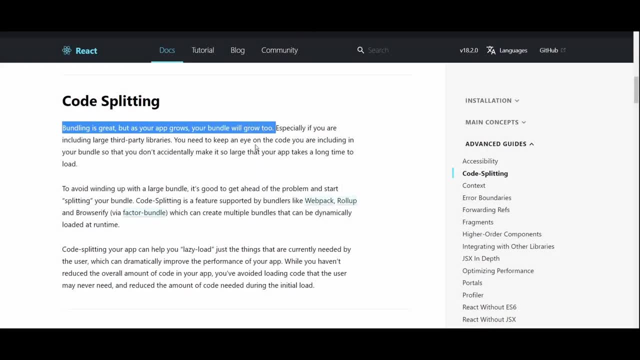 Code splitting in React is a technique used to split a large JavaScript bundle into smaller, more manageable chunks. It helps improving performance by loading only the necessary code for a specific part of an application, rather than loading the entire bundle up front. When you develop a React application, all your JavaScript code is typically bundled together into a single file. 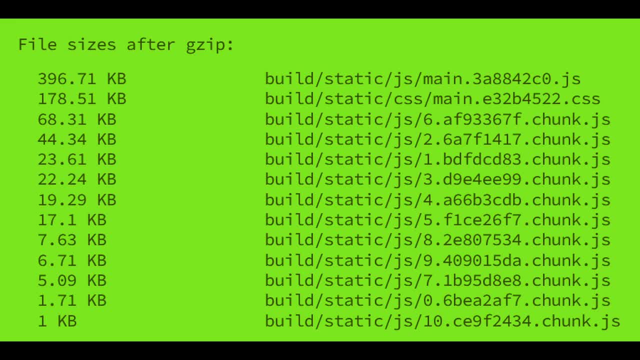 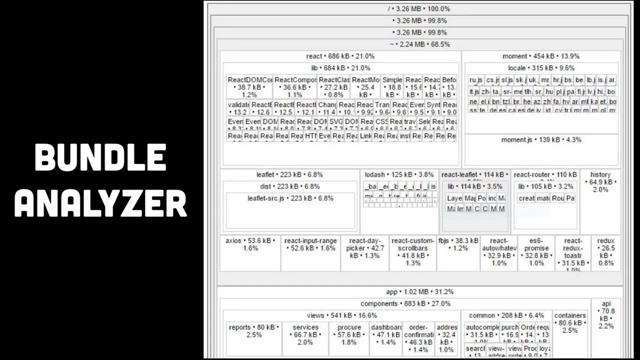 This file contains all the components, libraries and other code required for your application to function. However, as your application grows, the bundle size can become quite large, resulting in slower initial load times for your users. Code splitting allows you to divide this single bundle into multiple smaller chunks. 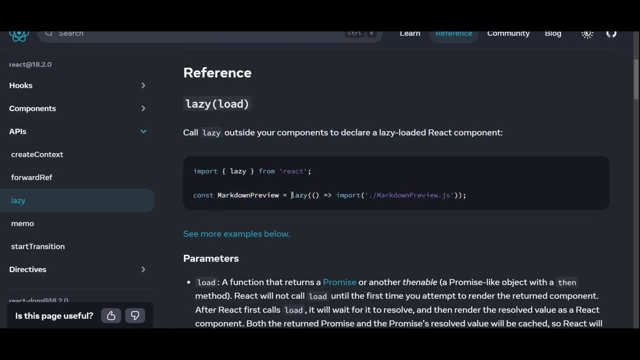 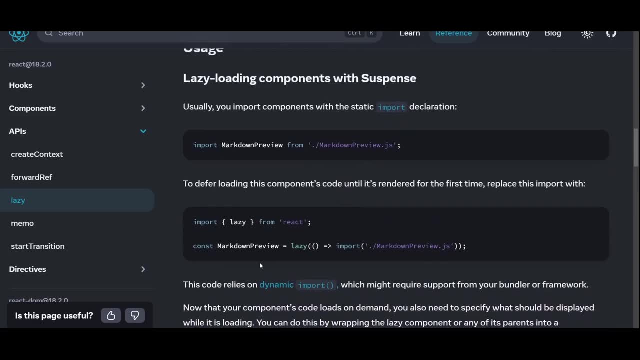 which can be loaded selectively based on the current needs of your application, Instead of downloading the entire bundle up front. only the necessary code is fetched and executed when a user visits a particular page or triggers a specific action. In number 6, there's React Fragments. 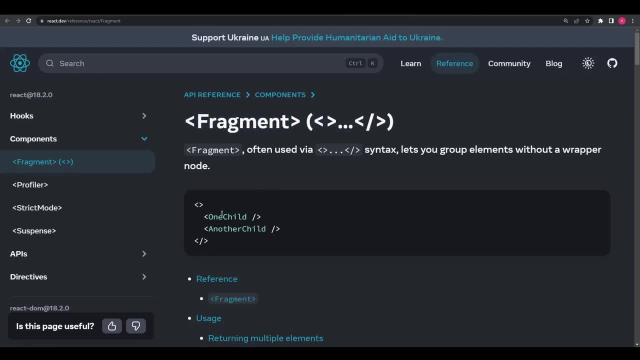 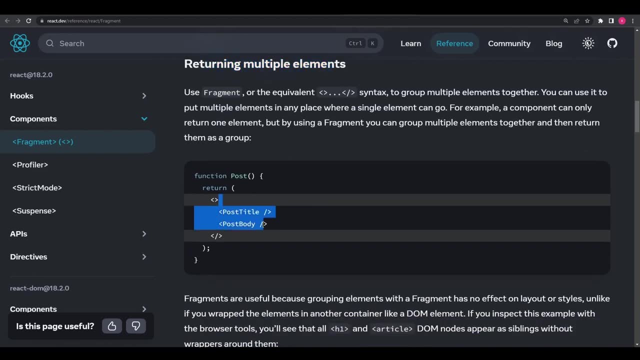 React Fragments allow you to group multiple elements together without adding an additional DOM node. They essentially reduce the number of extra tags and prevent extra DOM elements from rendering. When rendering a list of items or a collection of components, you typically need a parent container element to wrap them. 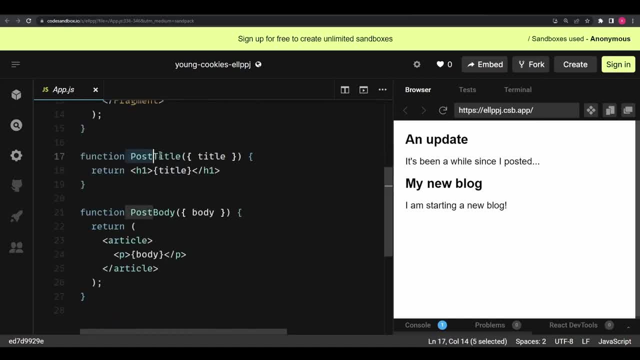 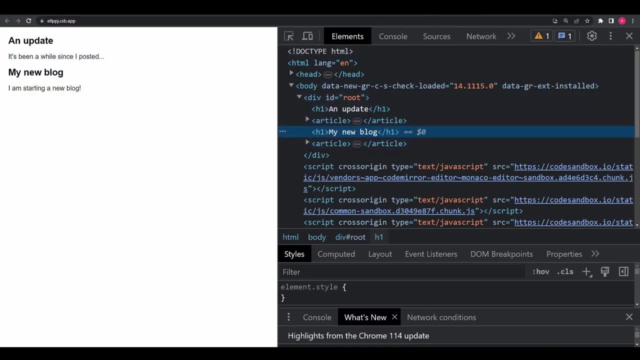 In such cases, using a React Fragment instead of a regular container element like a div avoids adding an extra node to the DOM, leading to a smaller DOM tree and improved performance. In number 7, we have WebWorkers. JavaScript is a single-threaded application.